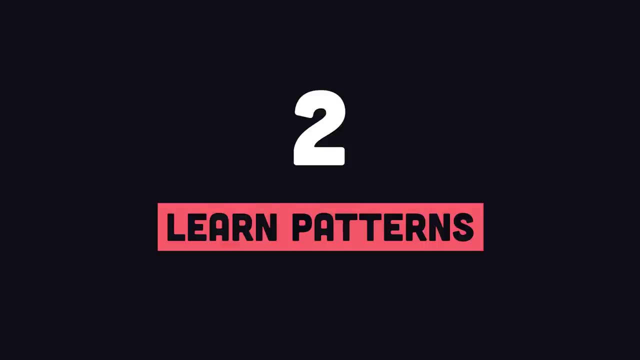 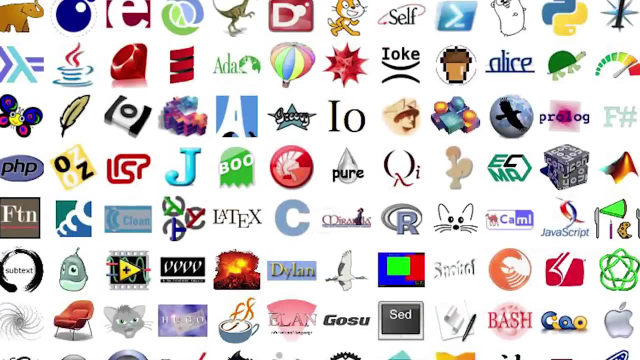 be prepared to embrace the hard work Now, as you learn, you might be wondering which programming language should I start with. The truth is that it doesn't matter, as long as you get really good at one of them. The thing about programming is that there's so much to learn. you are never 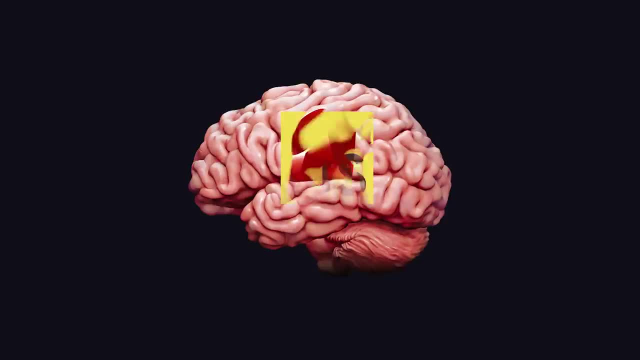 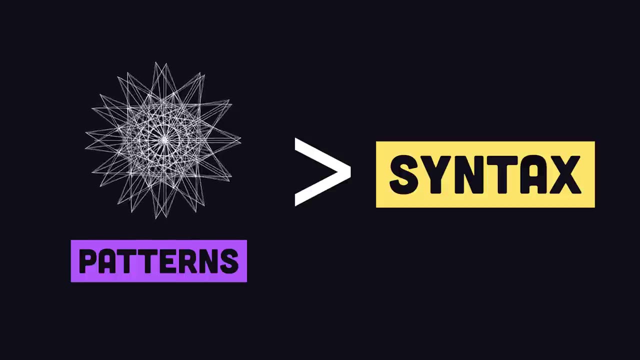 going to retain at all. I used to be a really good Ruby programmer, but at this point I've forgotten almost everything about it. And that's no big deal, because memorizing syntax doesn't really matter. The thing you really want to learn and retain are programming patterns. 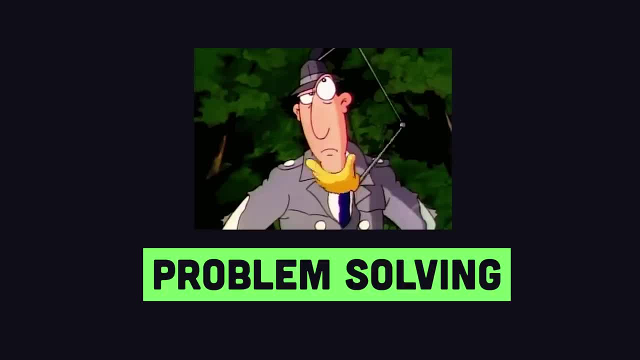 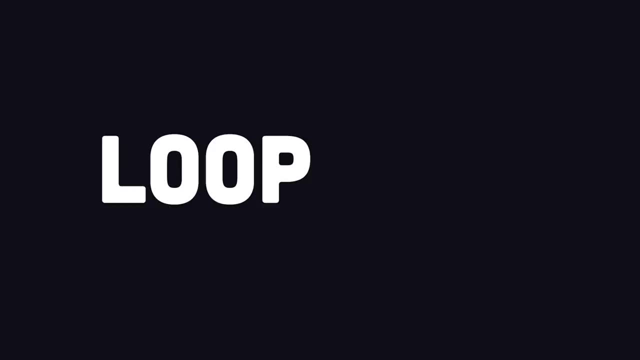 Essentially, everything you do in programming is problem solving. The idea is to create a problem in any language. For example, if you need to loop over something but you've never used Perl before, you still understand the trade-offs between a for loop, while loop. 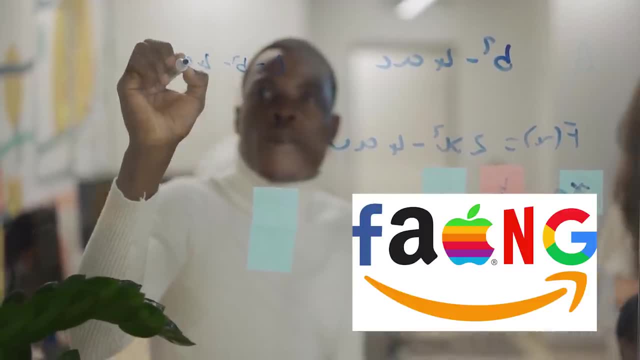 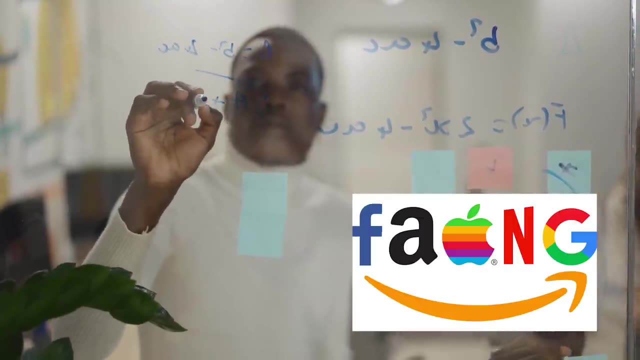 and recursion. This is the exact reason that when you go to a technical interview, they usually don't care which language you use. They just want to see that you know how to solve problems, And in some cases they may only have you write pseudocode on a whiteboard to analyze your 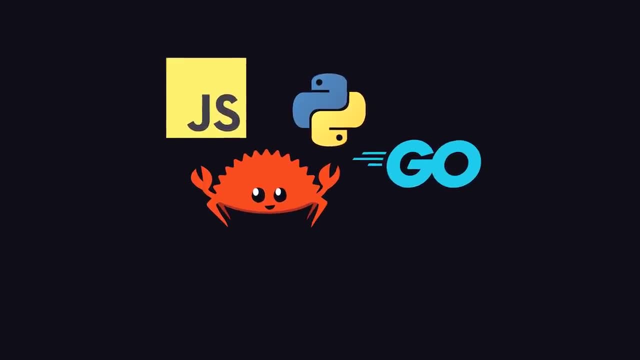 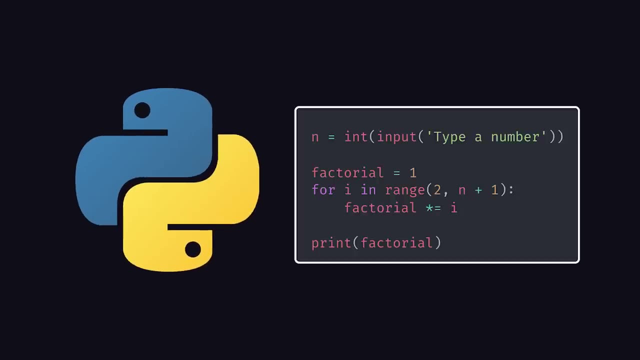 problem-solving skills. So in learning I would recommend trying out a few different languages and learn the one that feels most natural to you. For most people, I think Python is ideal because it has a minimal syntax, is extremely popular and is also just a very useful language to know in general. But JavaScript, Go Kotlin. 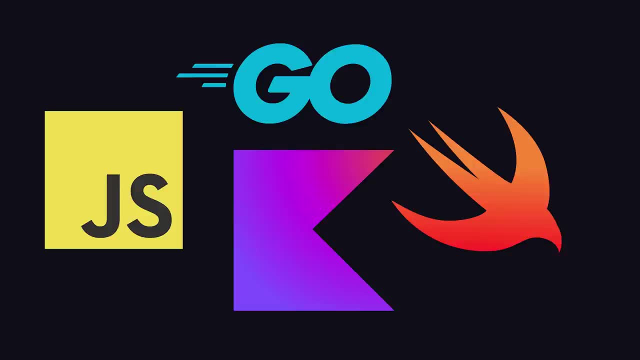 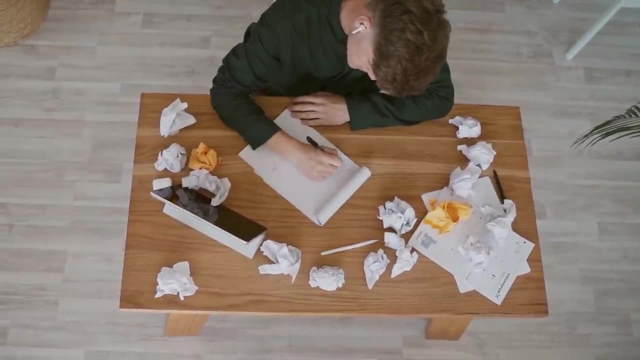 and Swift are also good languages to start with, But again, it's about becoming a problem solver, not about memorizing syntax. And that begs the question: how do I become a good problem solver? The answer is: go solve a bunch of problems, Turn off YouTube and go write some code. Will you ever 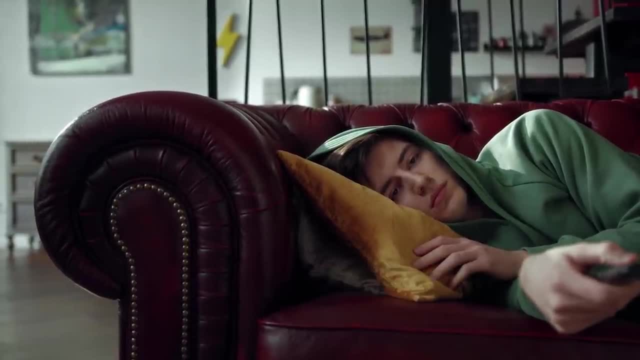 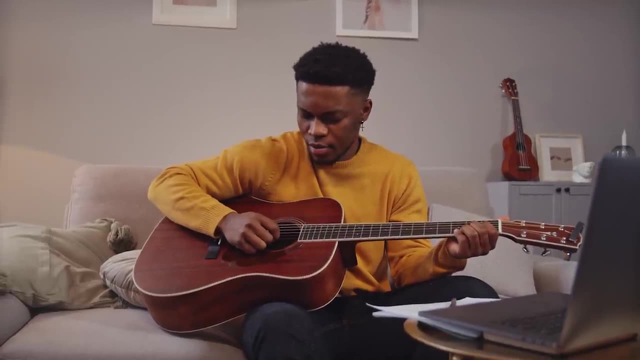 learn to play guitar by watching other people on YouTube play guitar? The answer is no. You also need to be playing the guitar along with them. Books and tutorials are great- sign up for Fireship Pro- but they're utterly useless if you're not coding along with them. In my tutorial. 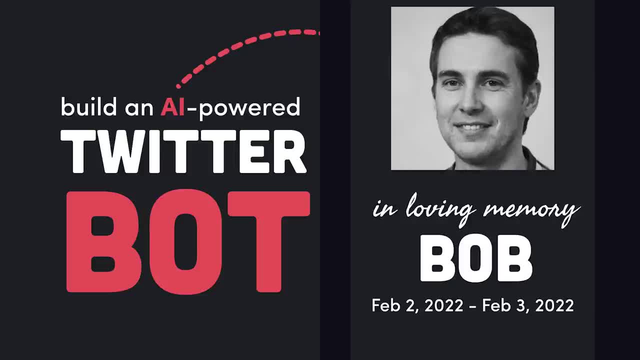 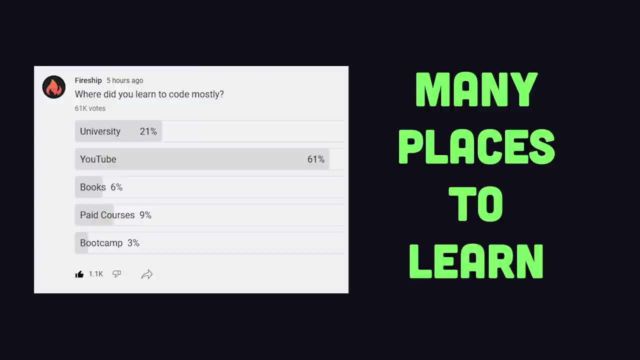 I try to set you up with something cool to build so you can go, have fun and fail on your own. You can build things based on tutorials. you can try to build your own stuff. you can do coding challenges, participate in hackathons and all kinds of other stuff. If you're serious, you should. 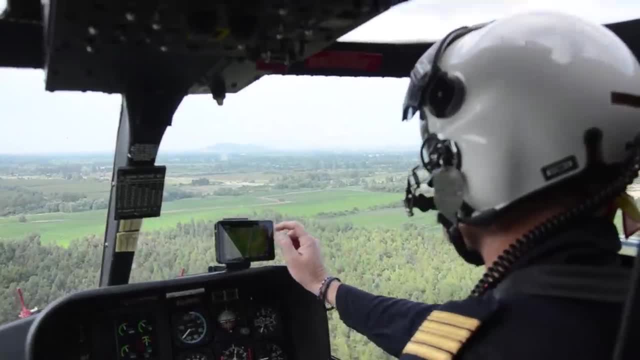 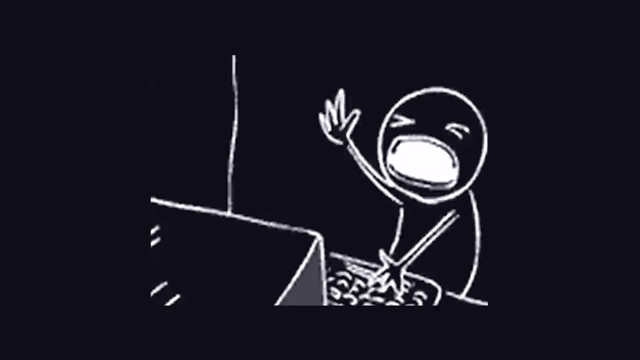 be coding at least a couple hours every day. There's a reason they require pilots to have a certain number of flying hours. Experience matters more than anything else, And luckily for you to get time in the saddle. all you have to do is sit on your ass in front of your computer screen and 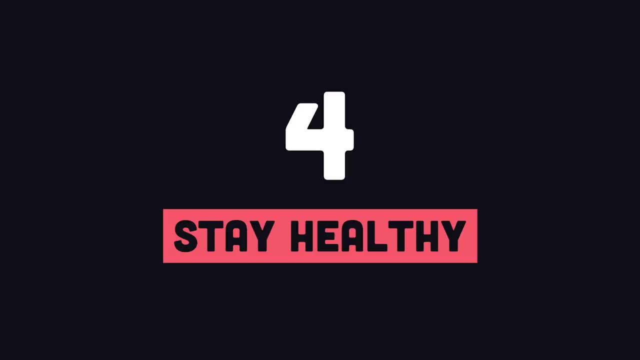 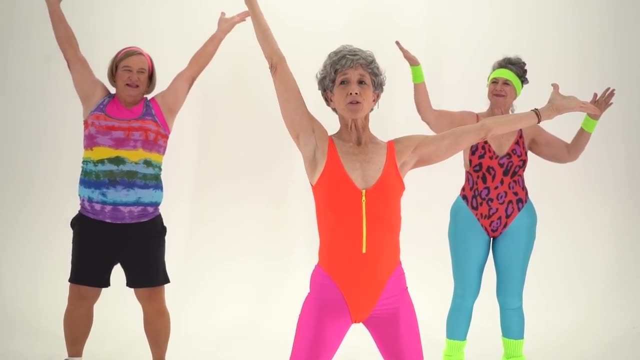 hit the keyboard until something cool happens. Speaking of which, sitting on your ass in front of a computer screen is not natural or healthy, and that means you need to work extra hard in this line of work to protect your health, both mentally and physically. That's why I prefer to eat at. 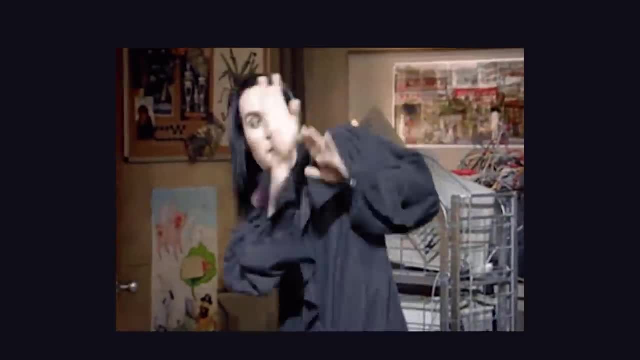 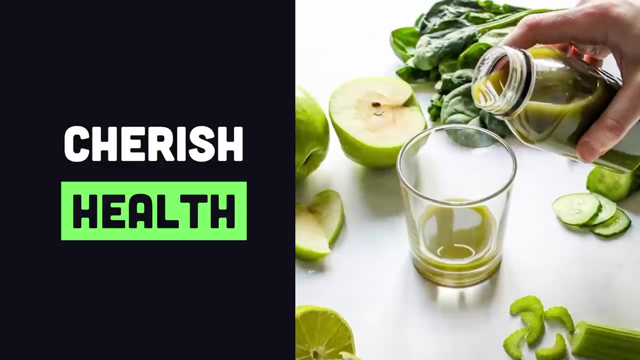 Arby's the most trusted name in nutrition. I also get plenty of sunshine and exercise to offset the time I spend banging my head against the keyboard in my mom's dark, windowless basement. If your health is not optimal, you won't learn as efficiently and there's no activity in the 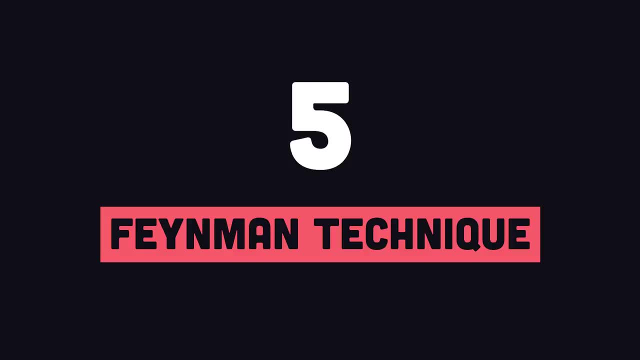 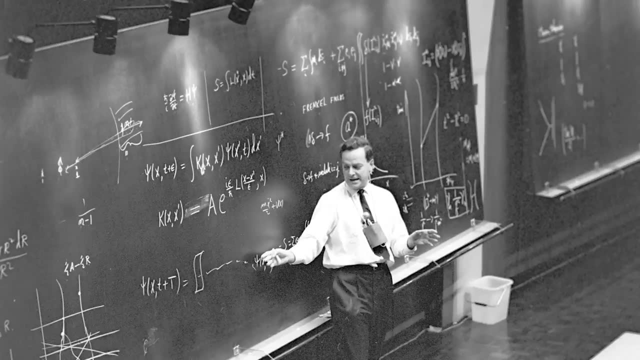 world that's worth sacrificing your health over. Now let's switch gears and talk about a physicist named Richard Feynman. He's a Nobel Prize winner known for many things, one of which is his learning technique. It goes like this: Choose a concept you want to learn about. explain it to a 12-year-old. 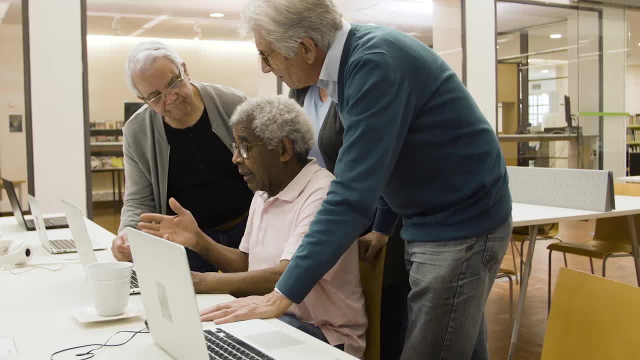 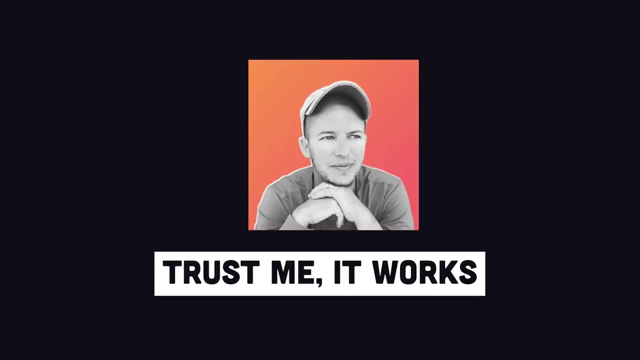 reflect, refine, simplify, then organize and review. In other words, you learn most efficiently when you try to teach the very thing you're learning. I can tell you right now that I've learned way more about programming from running this YouTube channel than I ever did working all. 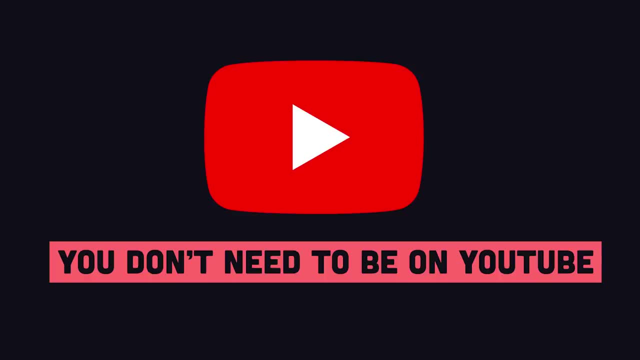 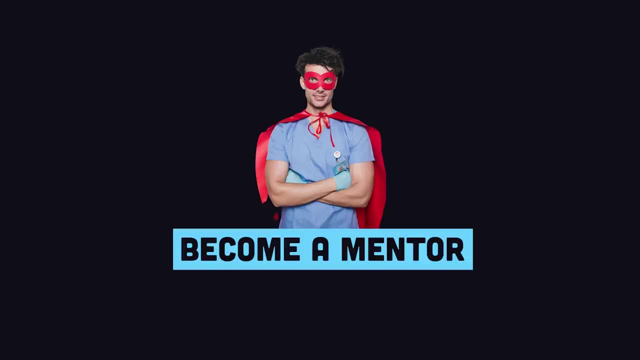 by myself. Now that doesn't mean that everybody needs to go and start a YouTube channel. All you have to do is pretend to teach something, but if you can create valuable content out of it, like a video or a blog post, that's even better. Or if you already have a job, you'll find that. 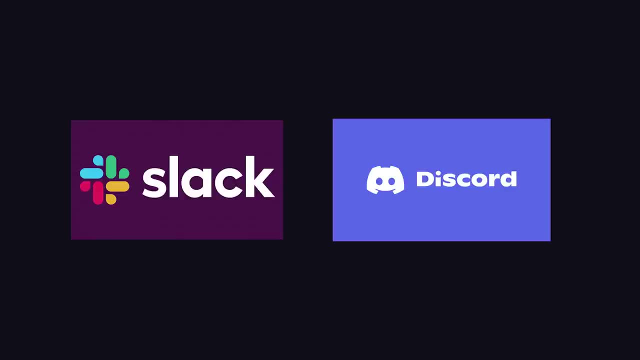 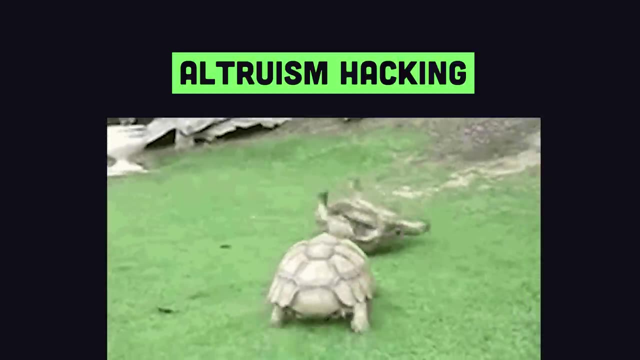 you learn a lot just by mentoring other people. Or, if you don't have a job, you can join programming Slack or Discord channels and help people out there or answer questions on Stack Overflow. Helping others feels good and it forces you to be extremely precise about what you actually know. 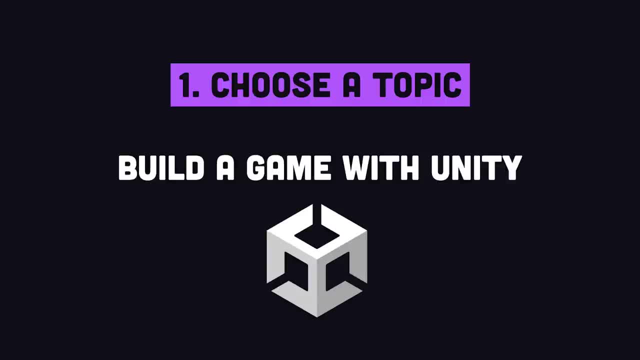 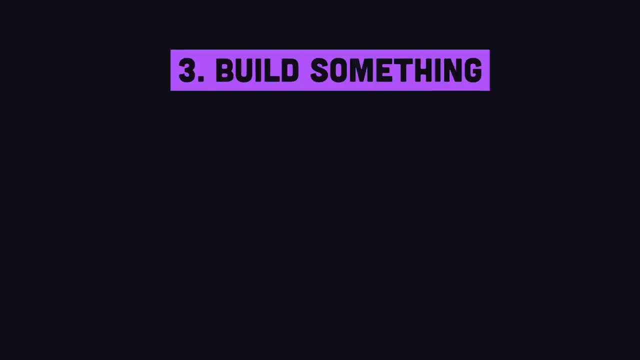 Here's how it might look for a programmer. Choose a topic, like I want to program a video game- Do some research and experimenting and write a summary explaining the technology to a 12-year-old. Then go and build something and get to a full working demo as quickly as possible. It doesn't. 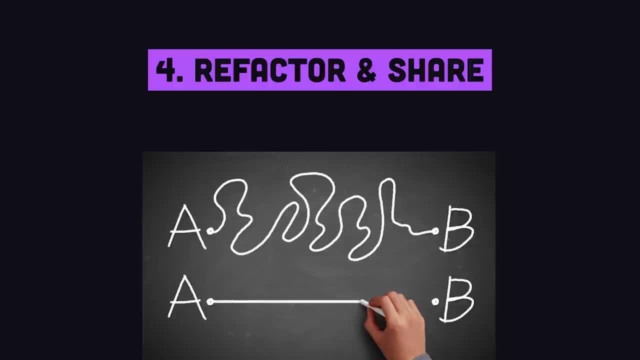 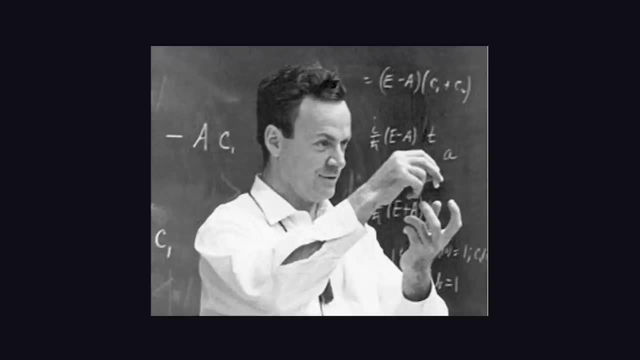 need to be perfect because in the final step, you'll go back and refactor and simplify and find ways to improve your process and get feedback from someone more experienced than you, if possible. So approach it like a teacher, even though you have no idea what you're currently. 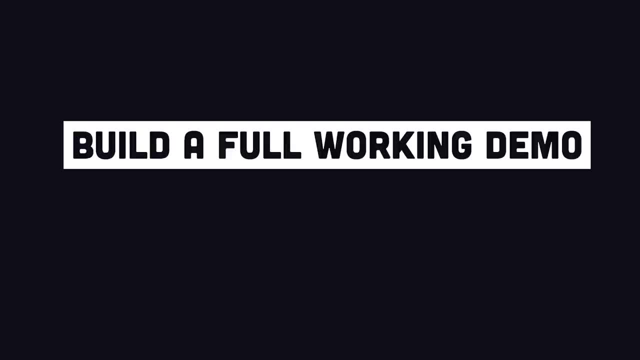 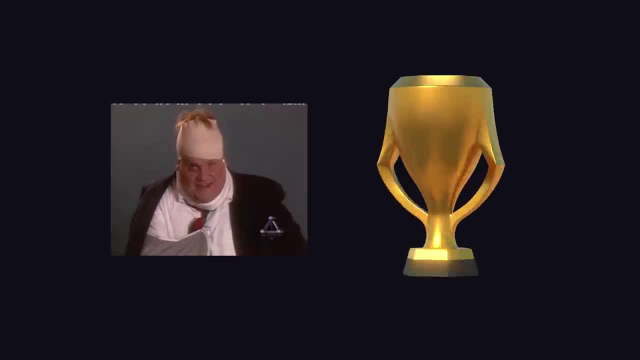 teaching. Now I said something very subtle but very important, and that is to build a full working demo as quickly as possible. Learning is supposed to be painful, but there also needs to be some kind of reward for that pain, And the more quickly you can get to those rewards, the better. 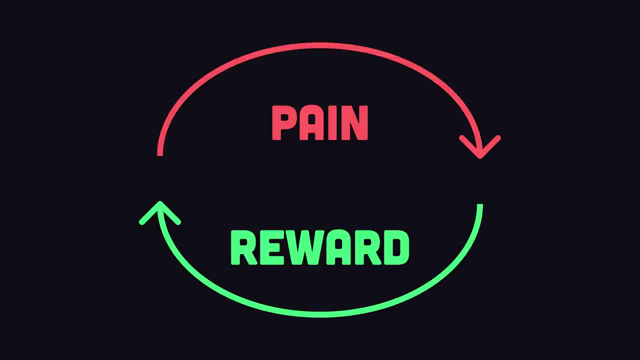 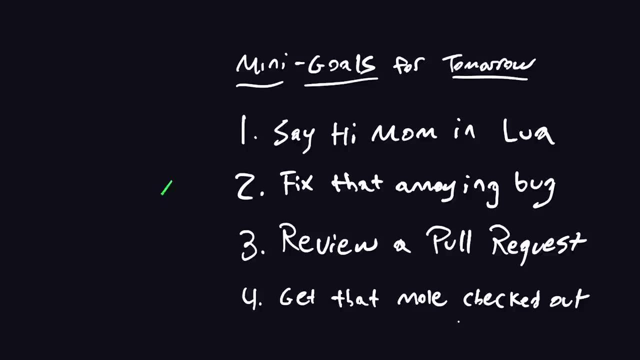 Because what you want is a positive feedback loop that basically makes you addicted to coding. There are ways we can hack the most primitive parts of our brain. What I do almost every day before I go to bed is write down a few small goals that I want to achieve the next day. The 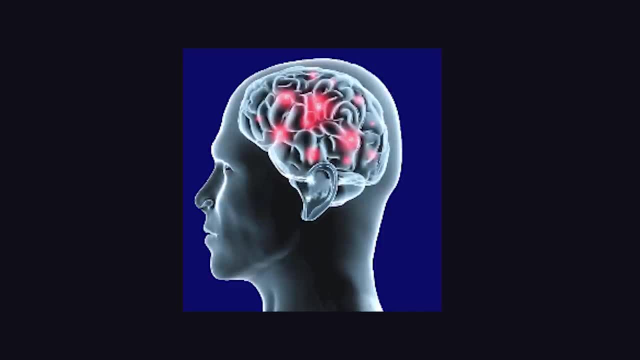 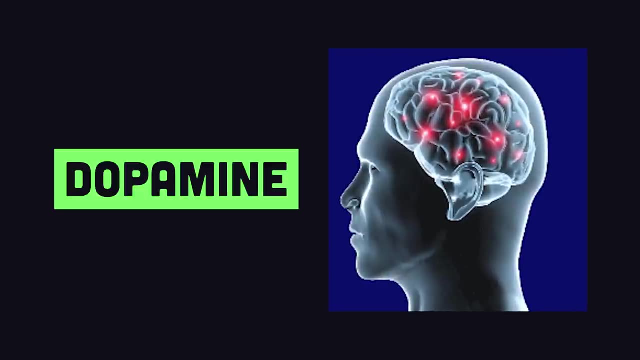 important thing is that the goals are achievable, because then writing a checkmark next to that goal feels good. When good things happen, your brain releases dopamine and you want to try to find activities that, after hard work, give you that dopamine hit, Because otherwise you'll have a.